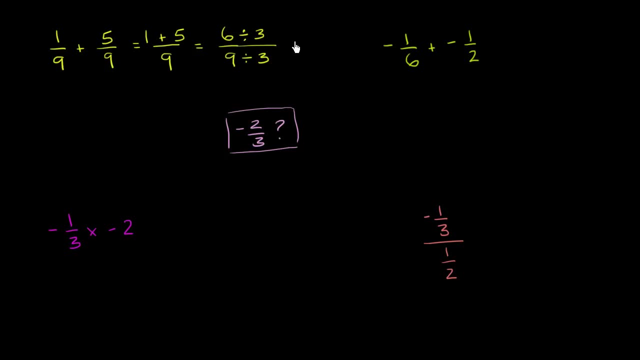 to get this fraction in a simpler form: 6 divided by 3 is 2.. 9 divided by 3 is 3.. So this is 2- 3rds, while what we're trying to get to is negative, Negative 2 3rds. 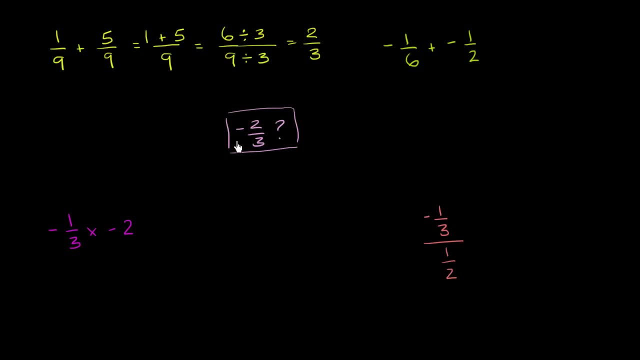 So these are not equal. This expression does not equal negative 2, 3rds, So I'll write no for that one. Now let's go to this green expression right over here. Give myself a little bit more real estate to work in. 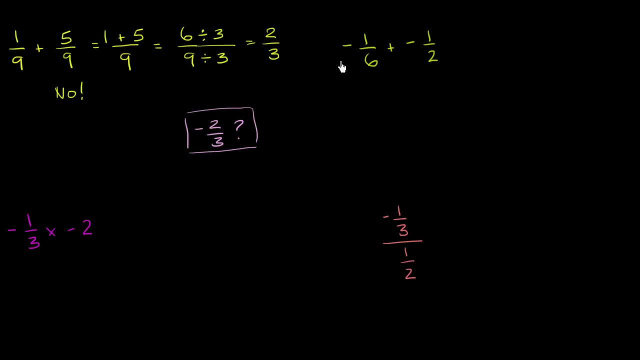 Now we have negative 1 6th plus negative 1 half. Now we can view this as being the same thing as. just to clarify, right now, the negative is in front of the entire 1 6th. The negative is in front of the entire 1 half. 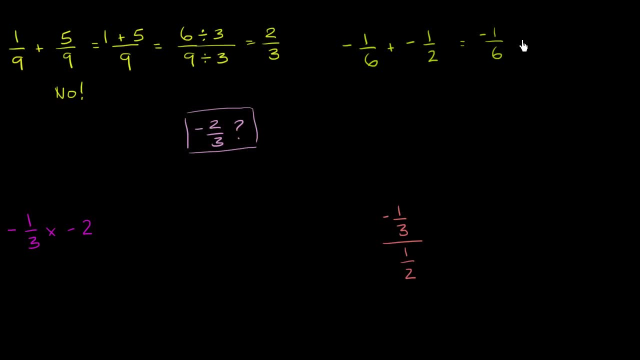 But this is the same thing as negative 1 6th plus negative 1 over negative, 1 over 2.. Negative 1 half is the same thing as negative 1 divided by 2 is one way to think about it And the whole reason why I did this. 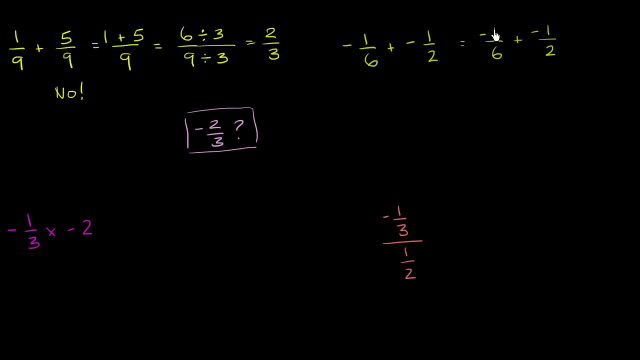 is. so we can simplify what the negatives are right now only in our numerator. So whenever we add two fractions, we want to have the same denominator And we see that 6 is already a multiple of 2. So we could leave this first fraction the way it is. 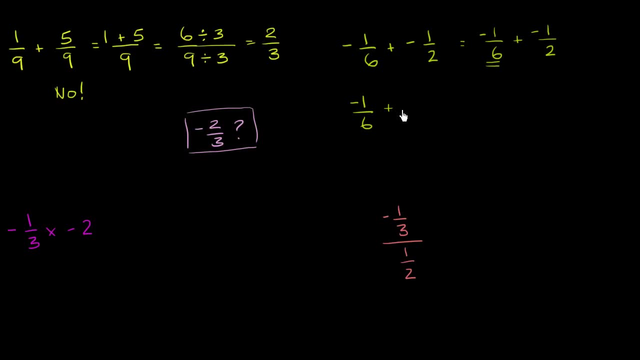 We can rewrite it as negative: 1 over 6.. And then the second fraction: we can write it as something over 6.. Well, to go from 2 to 6, we have to multiply by 3.. So let's also multiply the numerator by 3.. 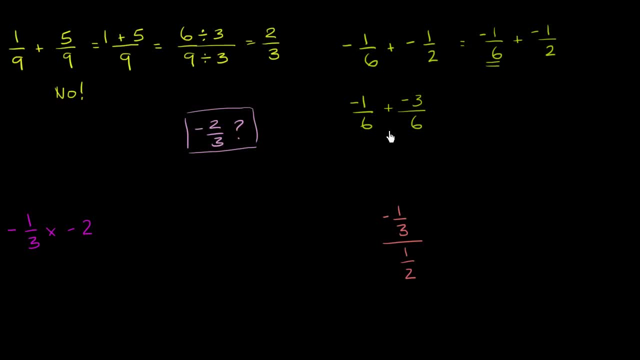 Negative 1 times 3 is negative 3.. So if I have negative 1- 6th and I add to that negative 3- 6th, this is going to be negative 1 plus negative 3- 6th, which 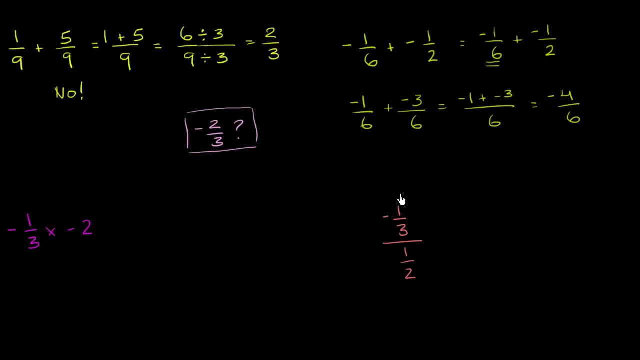 is equal to negative 4 over 6.. Now let's see if we can simplify. I guess we can even say: both 4 and 6 are divisible by 2.. So let's divide them both by 2. And in the numerator we're left with negative 4 divided by 2. 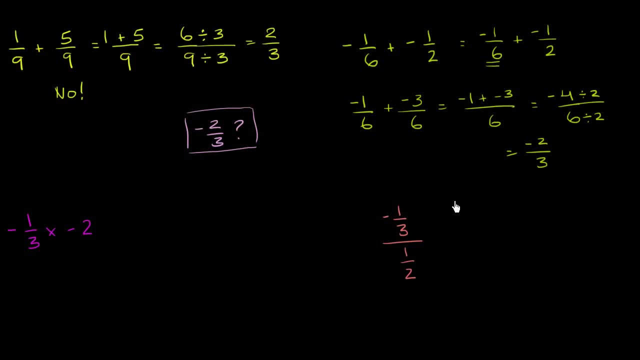 is negative 2.. 6 divided by 2 is 3.. Negative 2 divided by 3, well, that's the same thing as negative 2, 3rds, which is exactly what our goal value we're trying to get to. 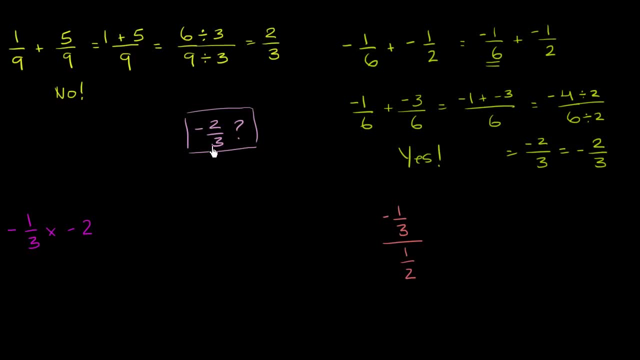 So, yes, this thing in green is equal to negative 2- 3rds. Now let's go over here. So we have negative 1- 3rd times negative 2.. Well, if you multiply a negative times a negative, we're going to get a positive. 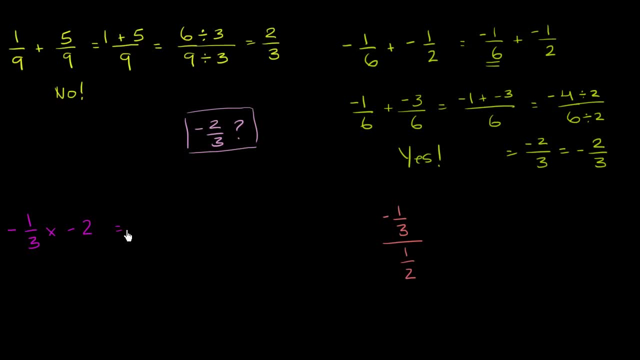 And we're going to get a positive 1, 3rd times 2.. So one way to think about it, this is going to be the same thing as 1, 3rd times 2, which is the same thing, And there's a couple of ways to think about it. 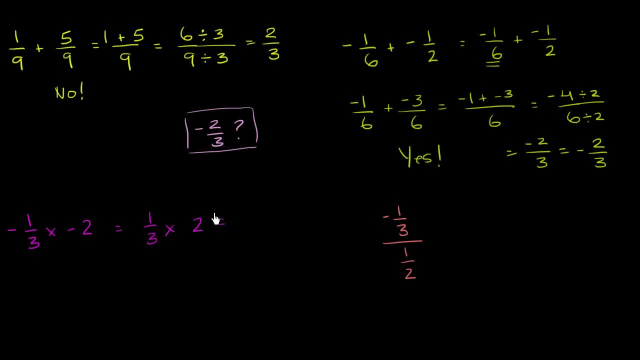 If you have a third and now you're going to multiply it by 2, you now have 2 3rds. Another way to think about this is that this is the same thing as 1 3rd times 2 over 1.. 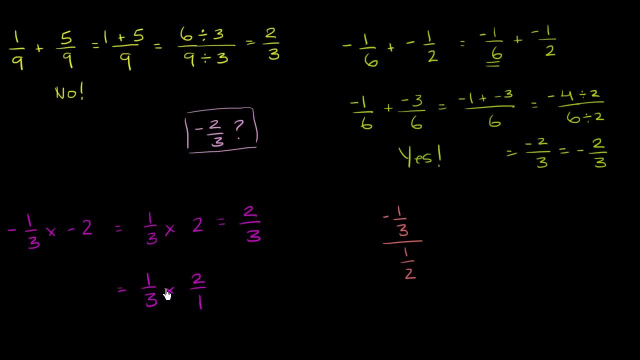 And you know that when we multiply two fractions- so this time we've expressed the 2 as a fraction- we can multiply their numerators, So it's 1 times 2 over the product of their denominators, 3 times 1, which is 2 over 3.. 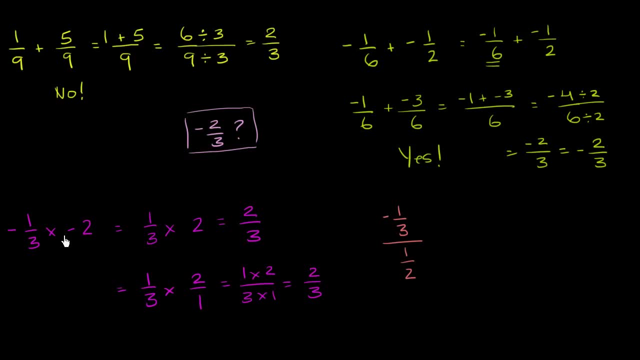 So, either way you look at it, this goes to positive 2 3rds. A negative times a negative is a positive. So it gets us to positive 2 3rds, not negative 2 3rds. So, like this first one, no, it does not equal negative 2 3rds. 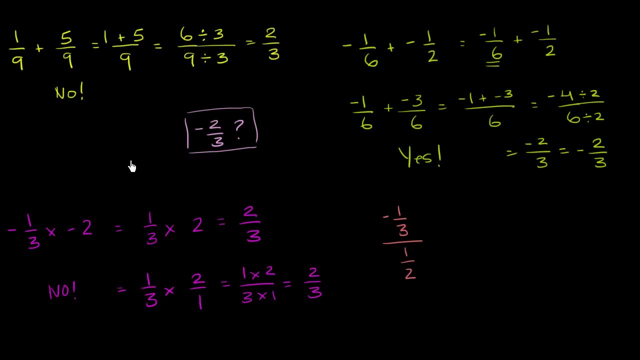 Now let's look at this one: Negative 1, 3rd divided by 1 half. So when you divide by a fraction, so when you take negative 1, 3rd dividing, let me write it this way: So negative 1, 3rd divided by 1 half. 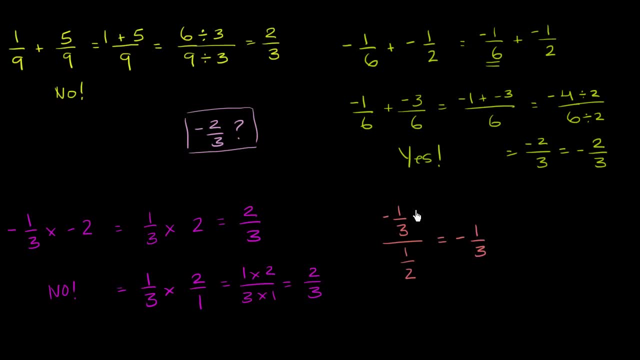 this is the same thing as negative 1- 3rd, And let me color code it just so you see what I'm doing. So let me make that green color, Let me make this a blue color. So negative 1- 3rd divided by 1 half. 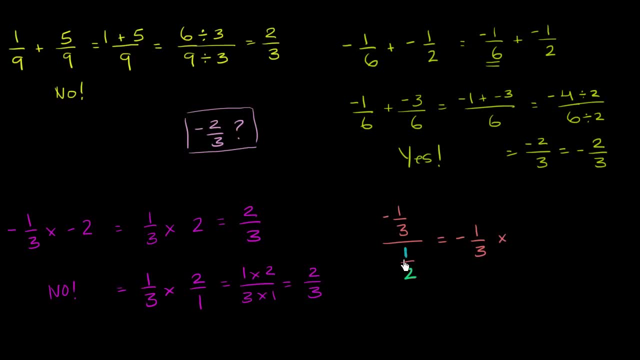 is the same thing as negative 1, 3rd times the reciprocal of 1, half, So times 2 over 1.. 2 over 1.. And what is this going to be equal to? Well, we can assume, instead of just viewing this: 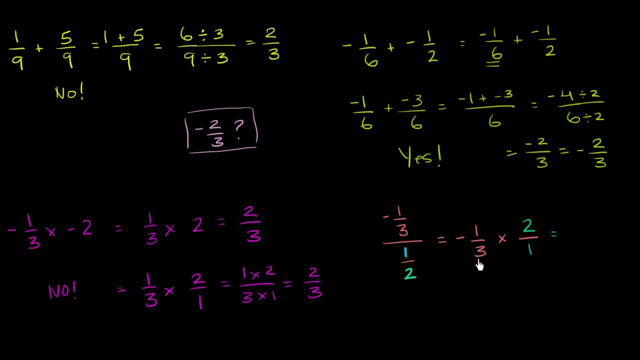 as negative 1- 3rd. we could view this as negative 1- 3rd. Negative 1 divided by 3.. That might help us keep track of the signs a little bit more, And so, if we do, this is- and let me actually- 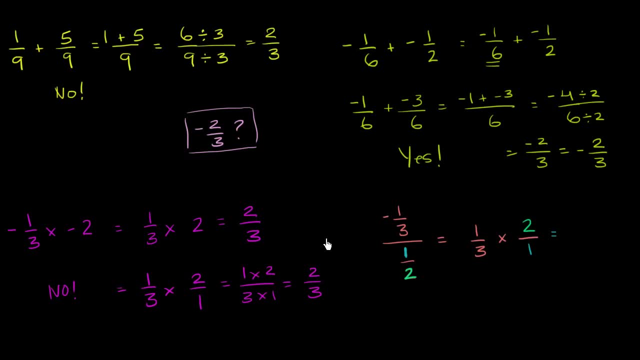 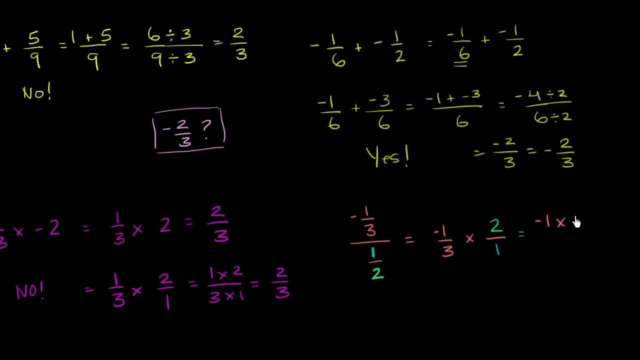 write it that way. just to make it a little bit clear, Let me write this as negative 1 divided by 3.. So our numerator is now going to be negative 1 times 2.. When you multiply two fractions, you just multiply the numerator. 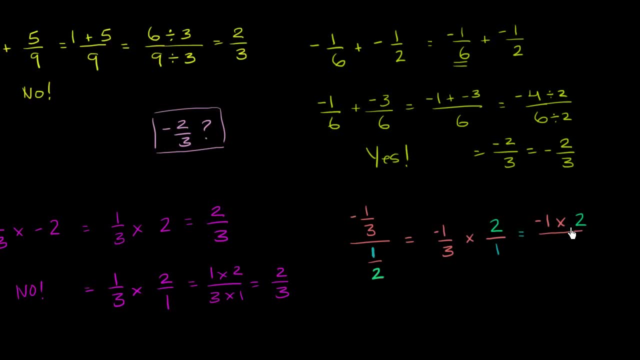 to get the new numerator, Multiply the two numerators to get the new numerator And it's over 3 times 1.. And you normally wouldn't have to do all of these steps, But I'm just doing them to make sure you understand what's going on. 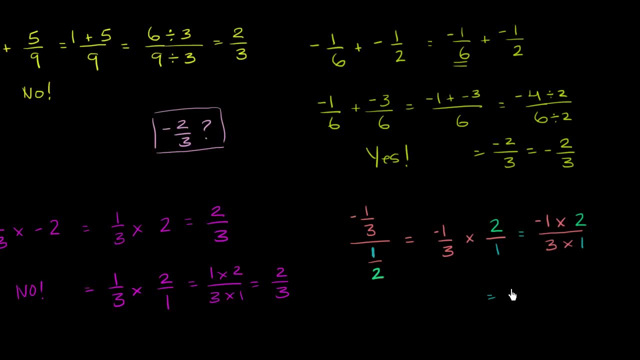 And so this is going to be equal to negative. 1 times 2 is negative 2. And 3 times 1 is positive 3.. Negative 2 over 3,- well, that's the same thing as negative 2. 3rds. 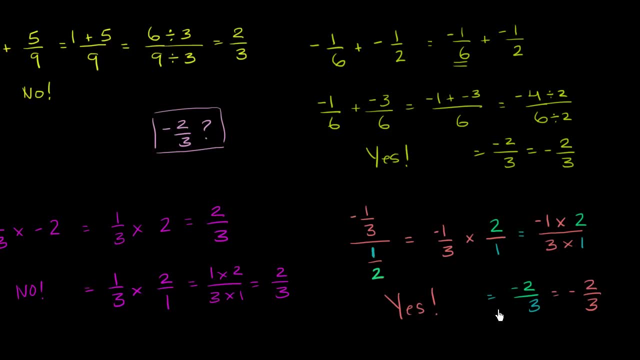 So this one works out: It is equal to negative 2- 3rds And it's going to be negative 2 3rds. 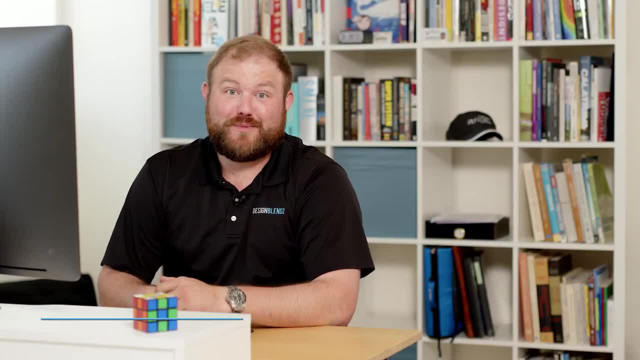 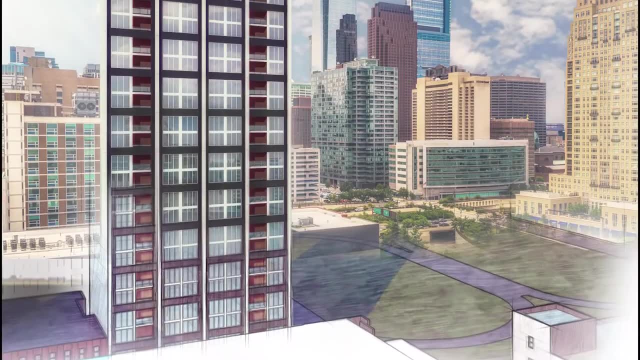 Architectural feasibility studies. It's the first step into any real estate project, whether you're looking to build something ground up or a renovation to a project. There are a few major things to look at in a feasibility study. One of the steps is space planning and area plans. Space planning and 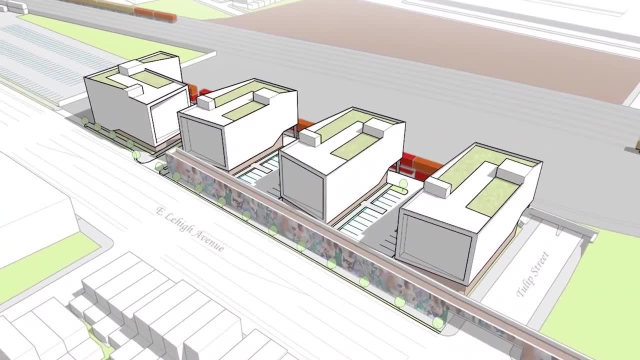 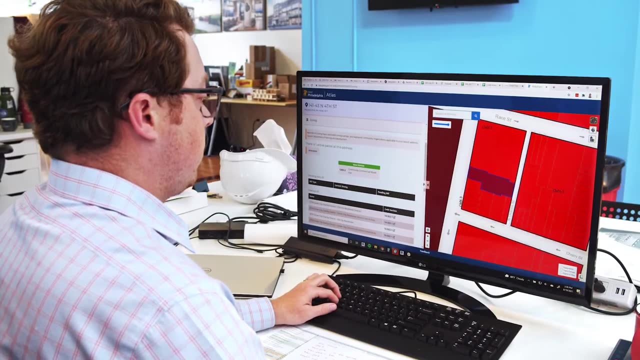 area plans ensure that we have enough space to meet project goals. We may be looking at unit counts, amount of commercial space or parking spaces in a potential project. We're also going to do a deep dive into the zoning code analysis, making sure that we've, you know, crossed our T's. 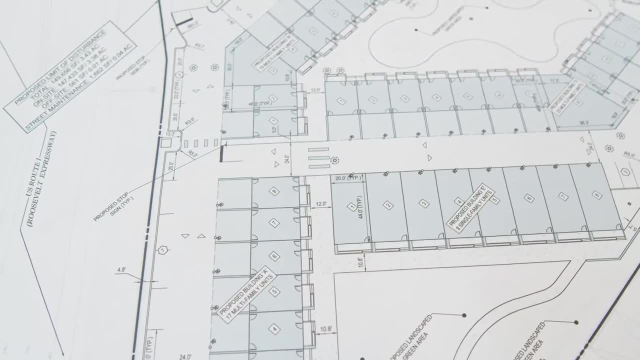 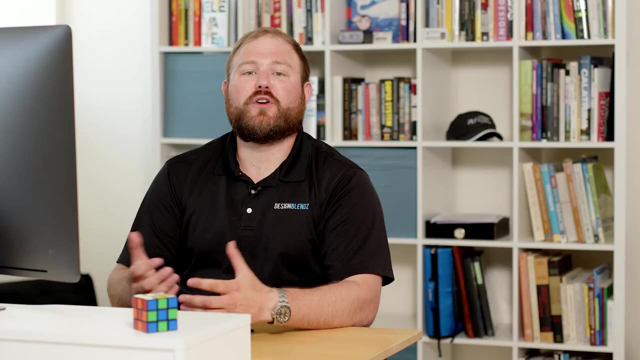 and dotted our I's certain things that play into that project and what's to come. Sometimes in the city there's properties that, based on where they're located, they have certain nuances and parameters around them. So if you're curious on what your project's full potential is from a